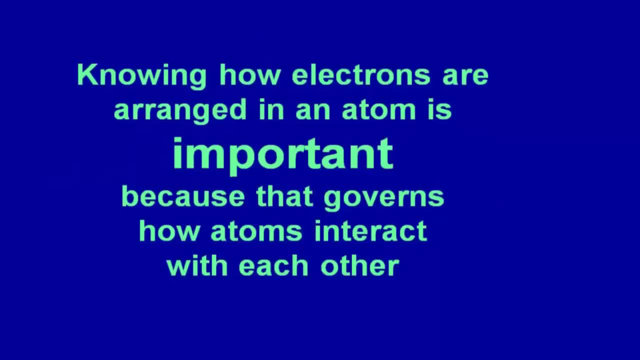 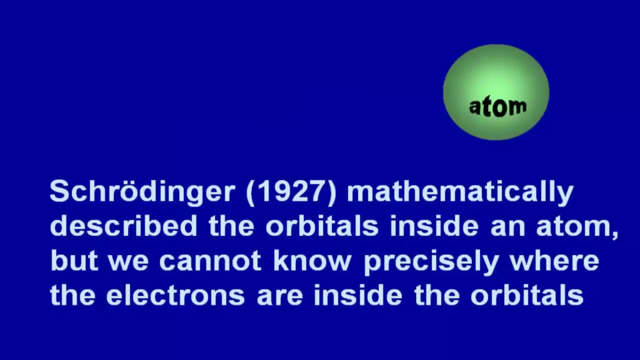 And that comes from Heisenberg's Uncertainty Principle And, as I said, this is important because the arrangement of electrons determines how atoms interact with each other. Schrödinger, building on Heisenberg's Uncertainty Principle as well as de Broglie's idea that electrons 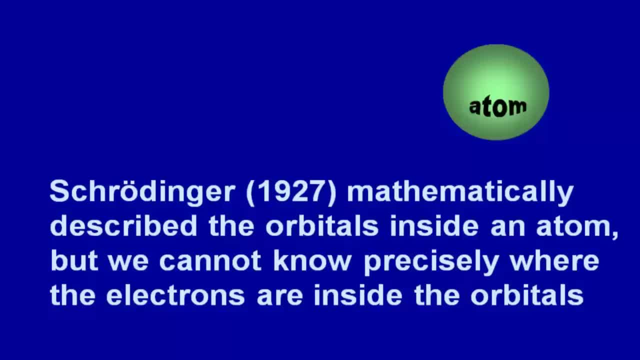 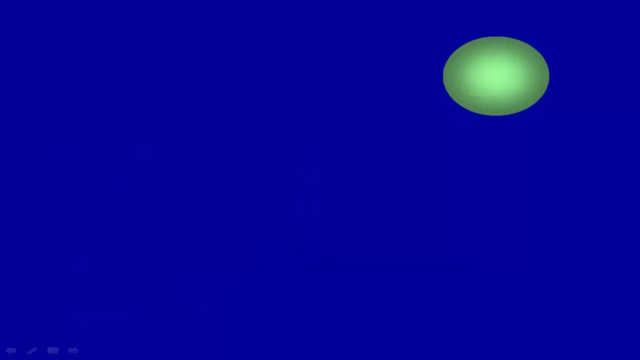 can act as waves. he created a mathematical model that described these orbitals inside an atom, these shapes, these high probability clouds. But we cannot know precisely where the electrons are inside the orbitals. And again, that comes from Heisenberg's Uncertainty Principle. 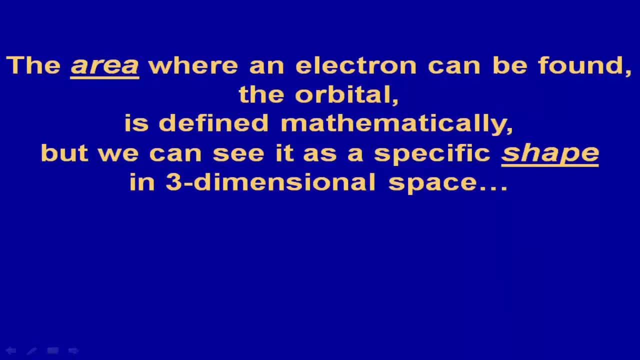 So the area where the electron can be found, the orbital, as we just said, is defined mathematically, But we can see it as a specific shape in three-dimensional space. So we're going to take a look at that three-dimensional space. 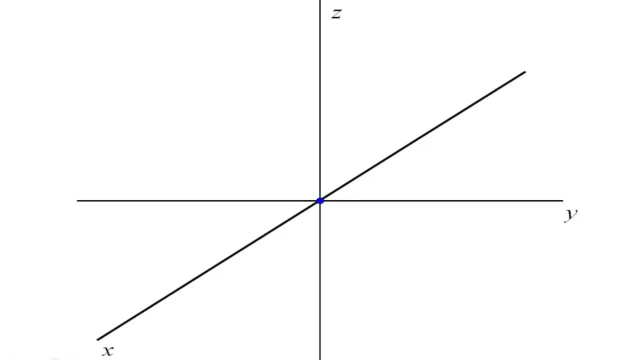 We're going to define it with the three axes x, y and z, the intersection of which will be our nucleus. Our first orbital is going to be the 1s orbital, And what we're going to do now is take a look at the shapes of orbitals and what they're called. 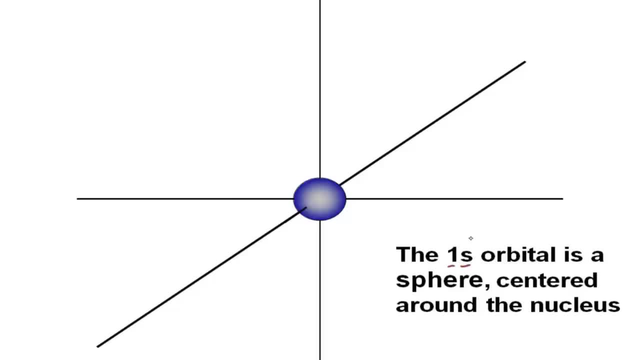 They're always designated with a number and a letter, And the letter designates the shape and the number designates the energy level. So the 1s orbital is the lowest energy orbital and the electrons in the 1s orbital are the lowest energy electrons. 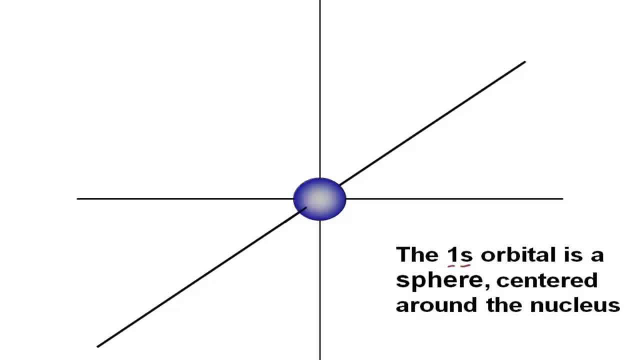 The problem is, orbitals can only hold a maximum of two electrons. So if we were talking about helium with two electrons, that would be fine. Helium would be happy with the 1s orbital. But what if we were talking about lithium? 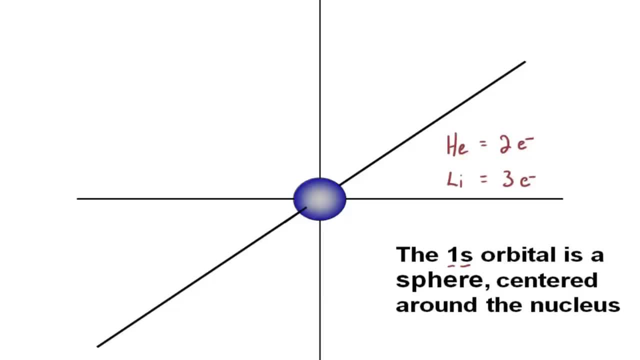 Lithium has three electrons. Where would the third electron go? Well, it would go in the next higher energy level orbital, which is the 2s orbital. Notice that we still have an s orbital And we still have a spherical shape. 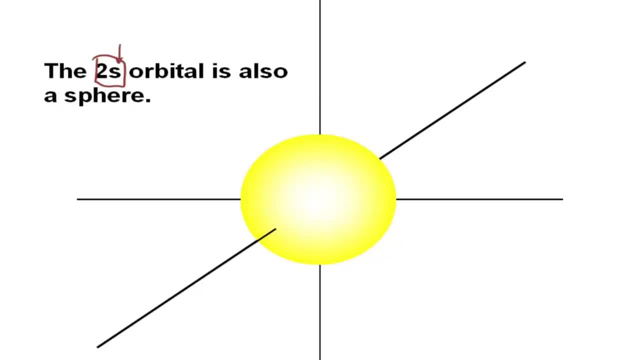 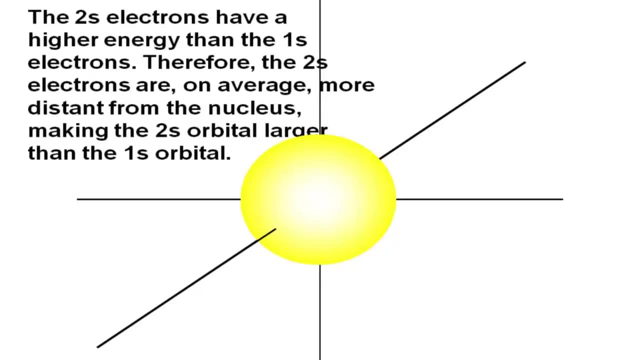 But the electrons in the 2s orbital are higher energy And so therefore, on average, they're going to be further from the nucleus, which describes, therefore, a larger shape, a larger area that they're going to occupy. But again, this is just a single orbital. 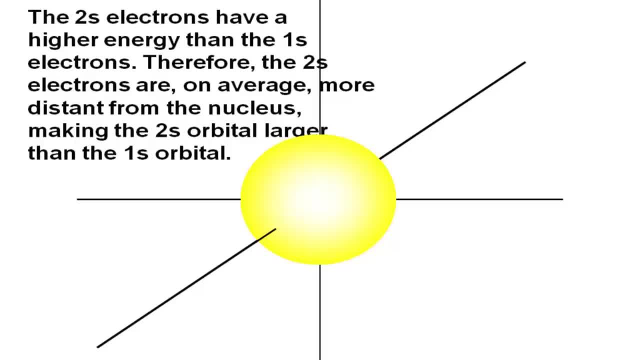 It can also hold two electrons. We still have the 1s orbital inside of it holding two electrons. So with the two orbitals we have now we can have a maximum of four electrons. That brings us to beryllium. So beryllium is happy with the 1s and the 2s orbital. 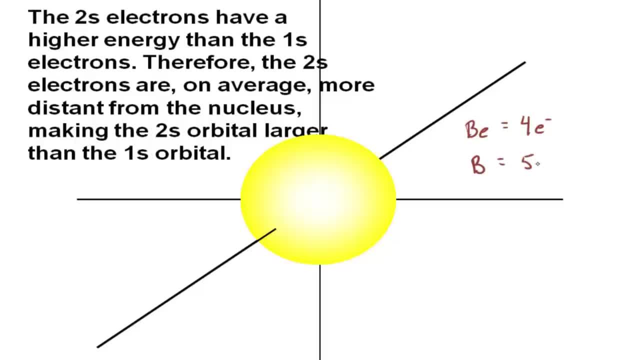 But what about boron? Boron has five electrons. Where is the fifth electron going to go? So, as you may have guessed, we're going to go to another orbital, a higher energy orbital, And here, just to review, we have the 1s orbital. 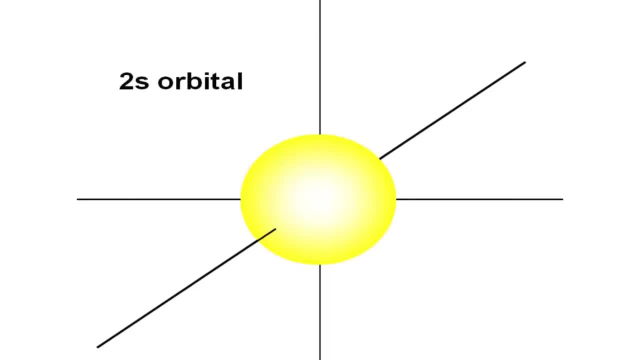 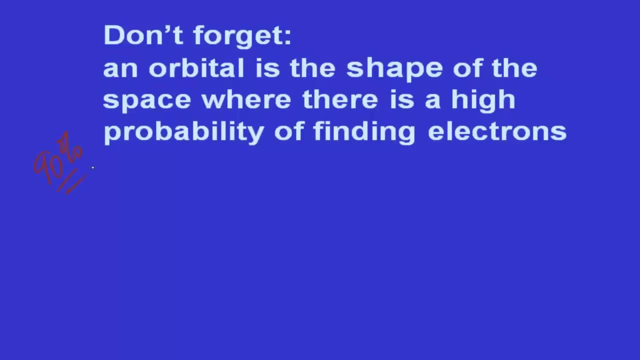 That has two electrons. We have the 2s orbital. That has two electrons. Don't forget, the orbital is the shape of the space where there's a high probability of finding electrons. 90% s orbitals are spheres. What about that fifth electron? 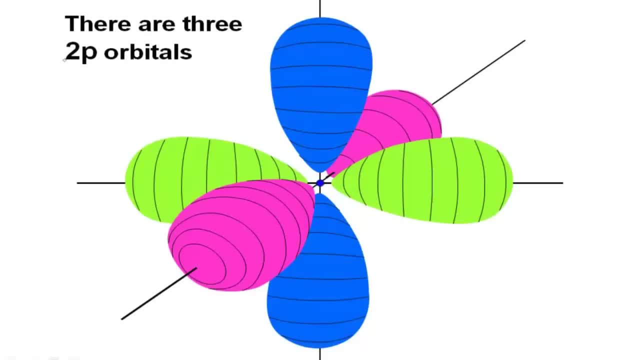 The fifth electron is going to start filling the 2p orbital. So here we have a different shape, Here we have the p shape And there are three 2p orbitals. They're all oriented perpendicular to each other, So we have this sort of pinkish red on the y-axis. 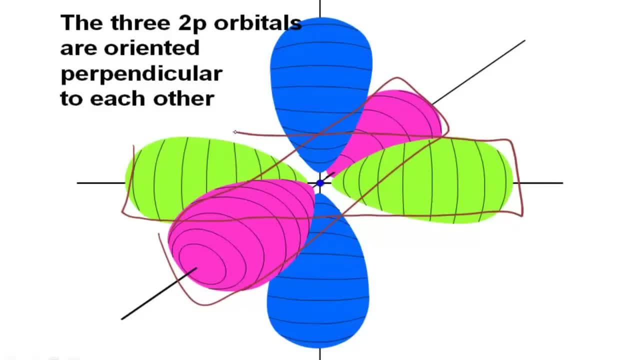 That's one orbital. Here's a second orbital along the x-axis, Sort of a greenish yellow I guess, And then the third 2p orbital along the z-axis. Now, each orbital, as you can see, consists of two lobes. 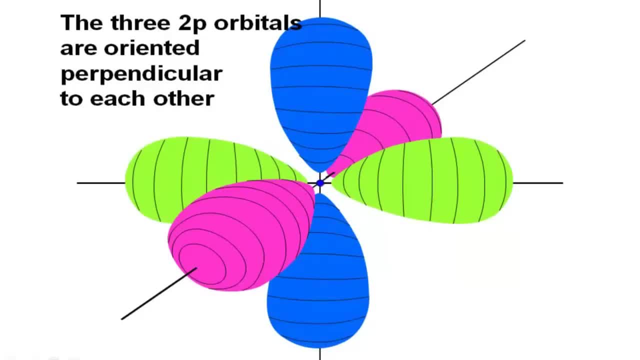 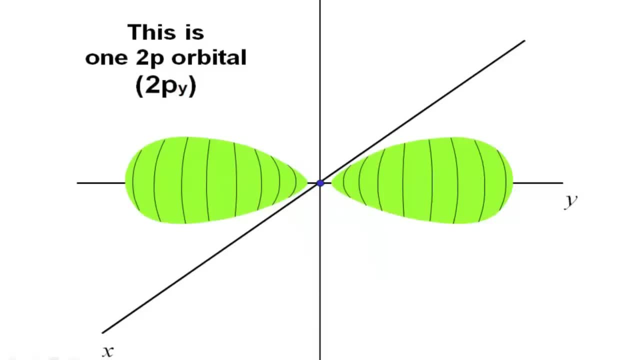 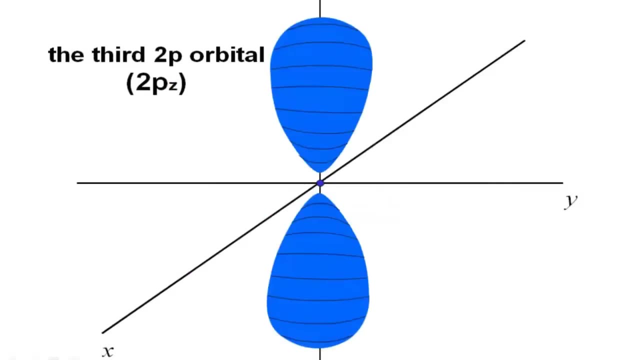 So both lobes together constitute just one orbital and can only hold a maximum of two electrons. So we designate each individual orbital by the axis it's on. So here the 2p orbital will be called 2py, 2px and 2pz. 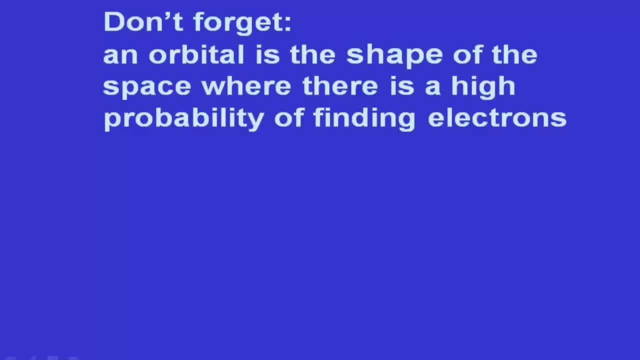 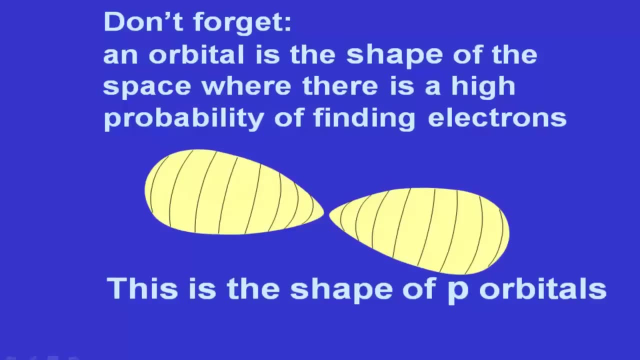 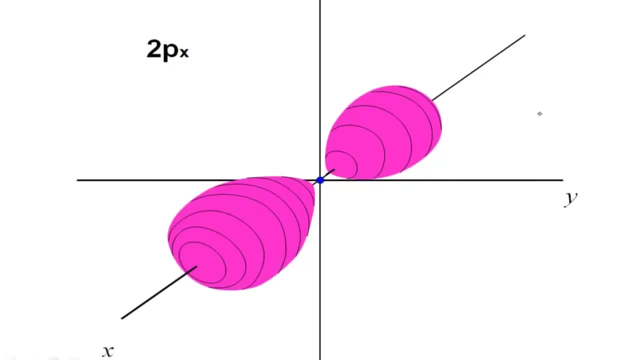 We cannot forget. the orbital is the shape of the space where there's a high probability of finding electrons, And the p orbitals. you could call them a dumbbell shape. They have two lobes. So let's say that fifth electron from boron goes into 2p. 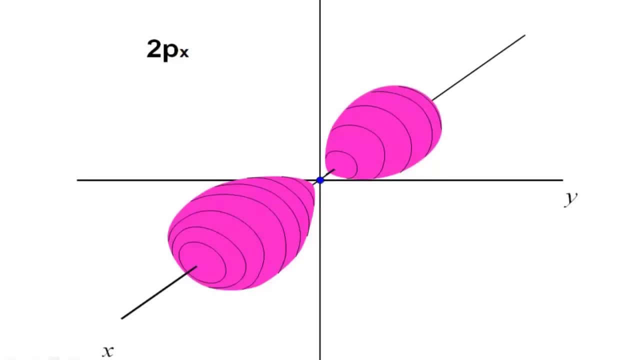 But what if we need to accommodate a sixth electron, which would be carbon? Carbon has a total of six electrons. Well, that could go into the 2pz orbital. And then what about nitrogen? The seventh electron that nitrogen has could go into the 2py orbital. 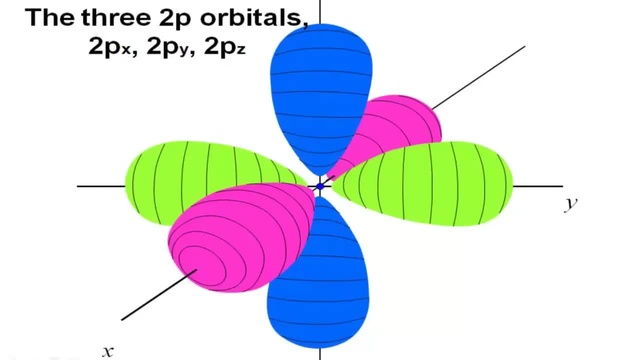 But we said that each orbital can have a maximum of two electrons. So once each of these orbitals has one electron, then they can start to pair up and fill each orbital with a total of two electrons And that would give the three 2p orbitals a total of six electrons. 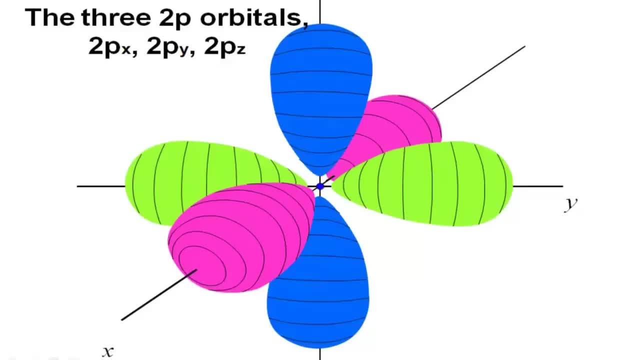 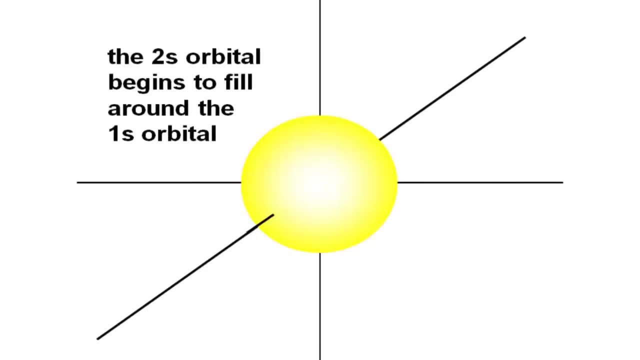 If the p electrons are filling up, we know that the 1s and the 2s must also be filled up. So let's take a look at that. Once the 1s orbital is filled, we can then start to fill the 2s orbital, but again with only two electrons. 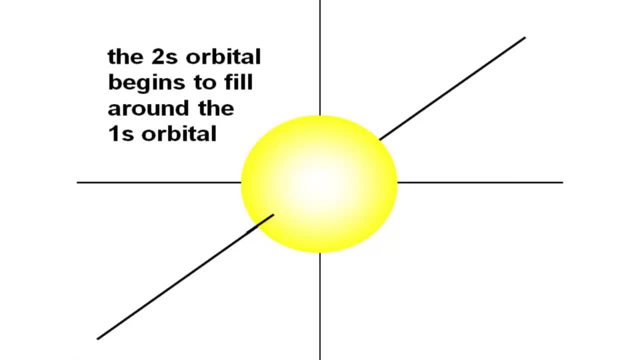 Once 2s is filled- and remember, 1s is still there, it hasn't disappeared. So 2s fills around the 1s. But now, once 2s is filled, we start to fill 2p Again, the 2s, the 1s. they're still in existence. 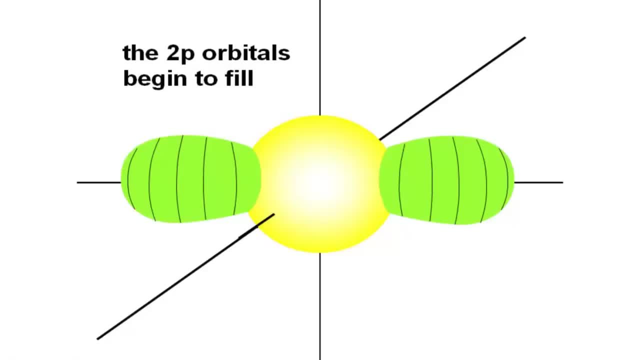 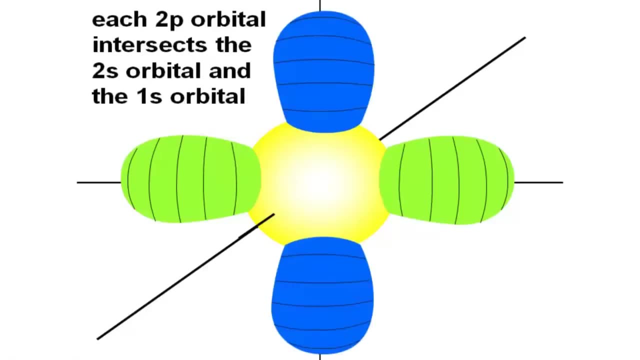 So therefore, the p orbitals actually overlap with the 1s and 2s orbitals. So here's one of the 2p orbitals. Once another electron would come and fill this 2p orbital. another electron would come and fill this 2p orbital. 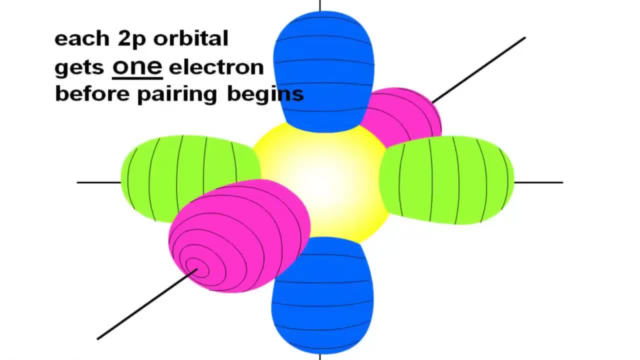 Let's say, all these orbitals are completely filled And therefore we would have the 1s orbital with two electrons, We would have the 2s orbital with two electrons And we would have the 2p orbitals with six electrons. 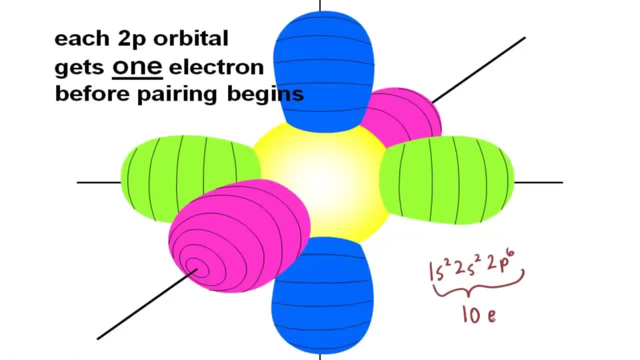 How many electrons total? is that Ten electrons? What element has ten electrons? Neon. So if all of these orbitals are filled up, that would be ten electrons and that would be neon. But what about sodium? Sodium has eleven electrons. 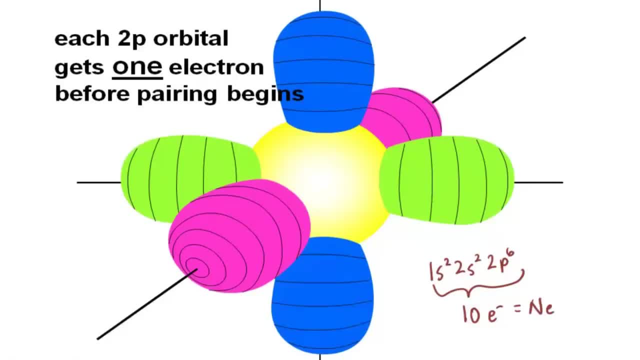 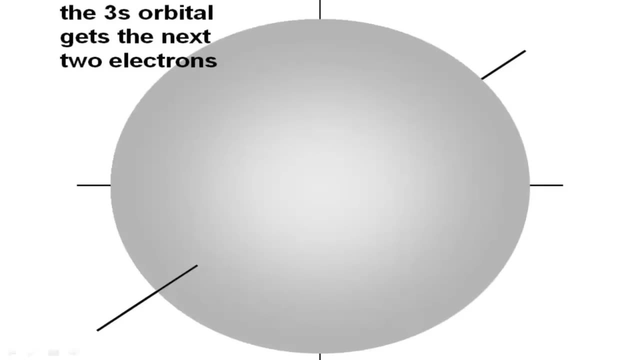 Where would that eleventh electron go? As you might have guessed, it would go on the next highest energy level, the next highest orbital, And that would be 3s. So 3s has electrons that have higher energy than any of those other orbitals we looked at. 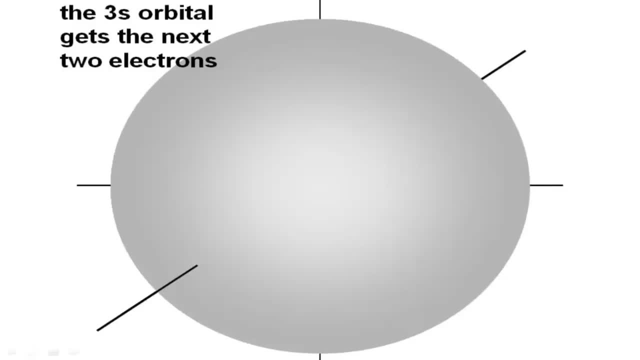 And so therefore the electron on average is further from the nucleus than the others And it is larger than 1s, 2s or 2p orbitals and surrounds them. So we can see the other orbitals still exist inside the 3s orbital. 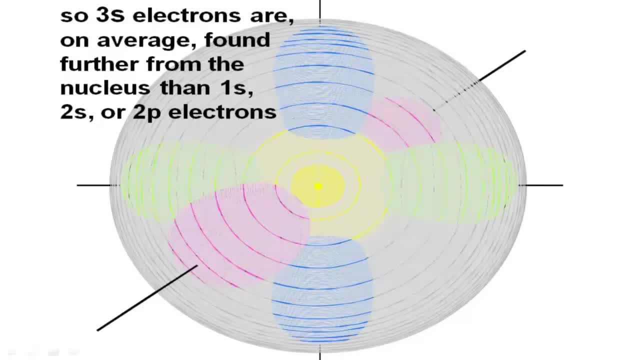 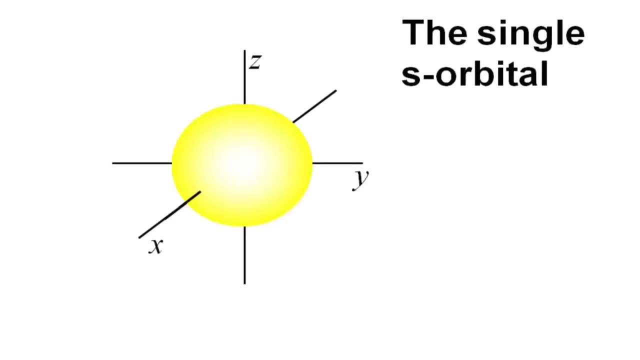 And the 3s orbital with sodium now is able to start getting electrons. So there's many more elements and there are other orbitals as well. So let's take a look at the other orbitals. First let's review the s orbital is spherical. 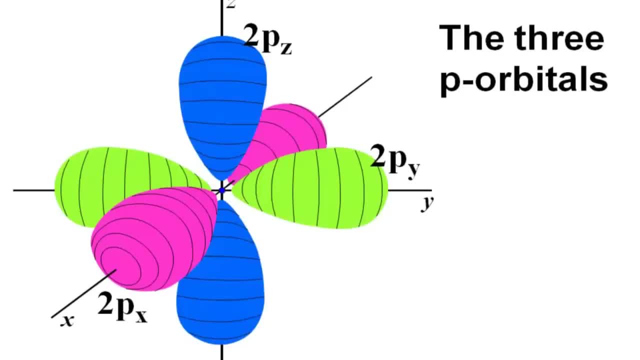 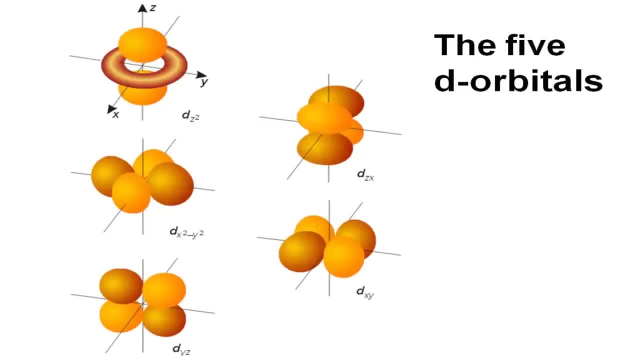 There's only a single s orbital at any one energy level. There's the 3p orbitals with this shape. There are 5d orbitals and this is their shape. So each one of these is a single orbital And each one of these can have at most two electrons. 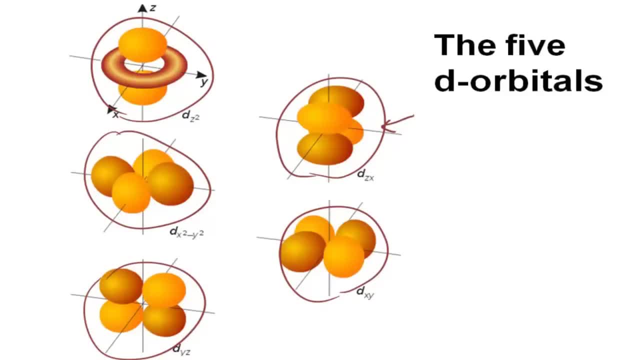 So they describe what we're looking at And the illustration describes the outer boundary of that 90% probability of where the electron is going to be. So that outer boundary, that surface that we're looking at, that surface plus all the space inside of it, constitutes the 90% area where we're going to find an electron in a d orbital. 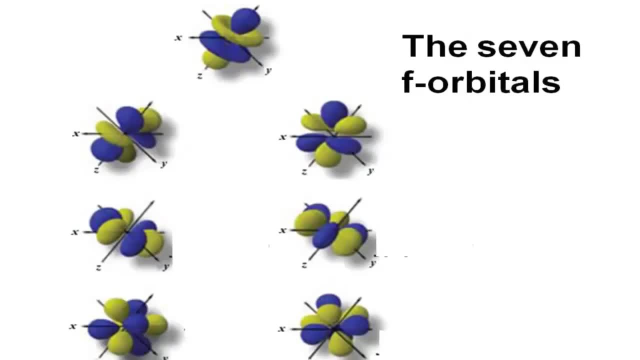 And then there's one more, the f orbitals, and there are seven of them Again. each one of these is a single orbital And each one of them can have a maximum of two electrons, So the electrons can be anywhere. They're traveling 90% of the time, anywhere inside these lobes. 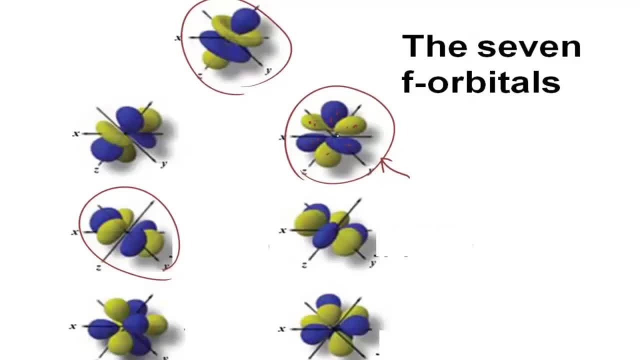 And if you track the electron long enough, you will start to see them describe these exact shapes that we're seeing here. One thing I think that students can get confused with is these shapes and what they represent, Especially when they get as complicated as the d and the f orbitals. 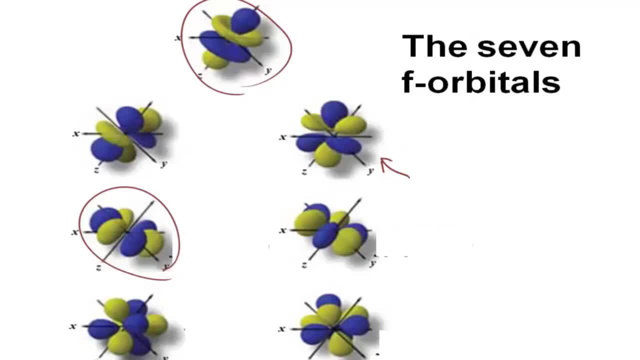 And there's even the g orbitals that are even more complicated than f orbitals. So don't get tripped up by the complicated shapes. All you need to really understand is what they represent, And they simply represent space, inside of which you're going to find the electron 90% of the time. 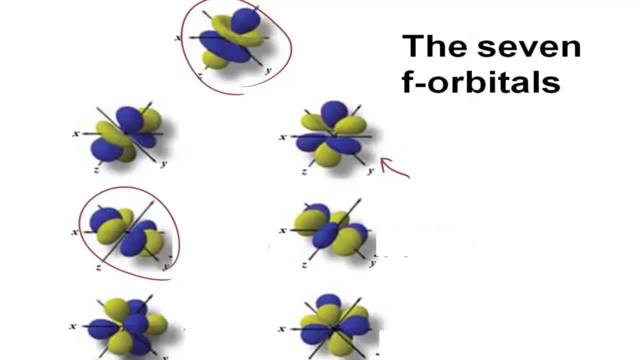 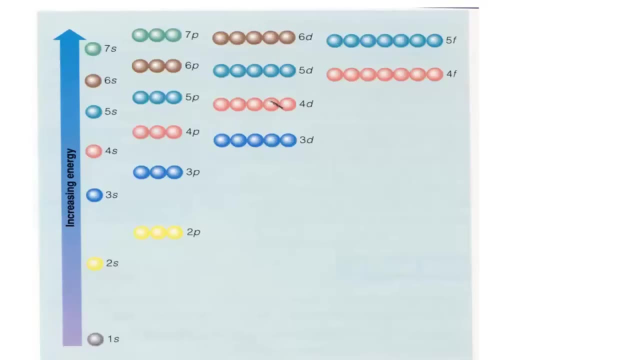 So you don't have to worry about the specific shape so much, Just know what these shapes represent, Where the electron is going to be. So, finally, a nice way to look at that is this kind of schematic: Energy is shown increasing on the y axis. 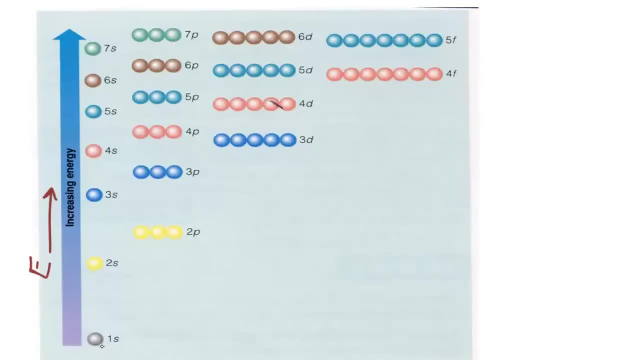 And each orbital is represented as a circle. The circles don't represent the shape of the orbital, They're just representing the existence of the orbital. So at any one energy level, there's always just a single s orbital, And so the s orbitals as you go to 1s, 2s, 3s, 4s, etc. 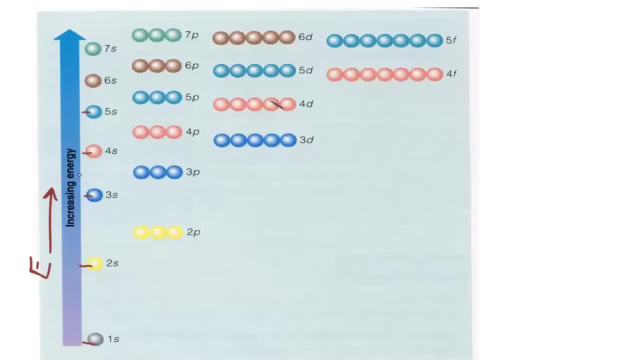 They keep increasing in energy. As we saw before, 2p orbitals are higher in energy Than 2s And there is 3 of them, So the 3 circles represent the 3 2p orbitals, Not the shape, just the fact that there's 3 orbitals within the 2p energy level. 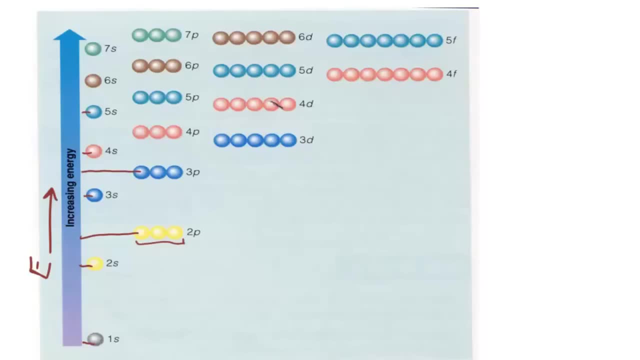 The 3p energy level. again, p always just has 3 orbitals. But what about d? We saw before that there are 5 d orbitals. So at any energy level that has d orbitals There's always going to be 5 of them at that energy level. 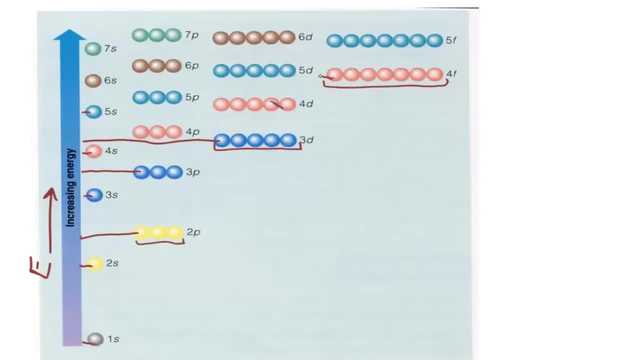 Then finally, f orbitals. There's 7 of them. So any energy level that has f orbitals is going to have 7 of them, As long as there are electrons to fill those orbitals, The orbital does not exist unless the electron is in the orbital. 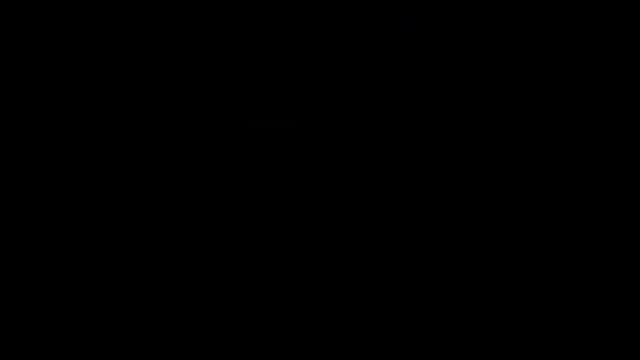 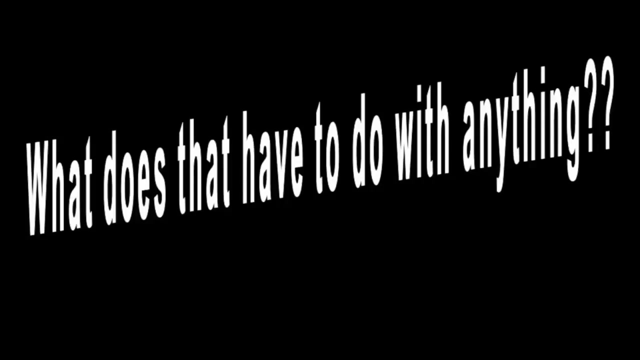 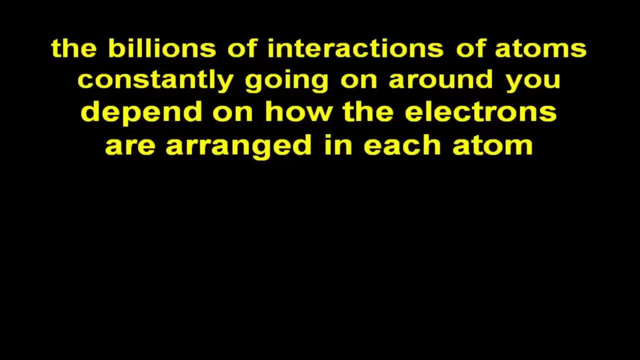 So what might you ask? Does that have to do with anything? Why do we care about how electrons are arranged in atoms? Well, atoms are constantly interacting around you, on the earth and the solar system and the universe. Those interactions depend on how electrons are arranged in each atom.